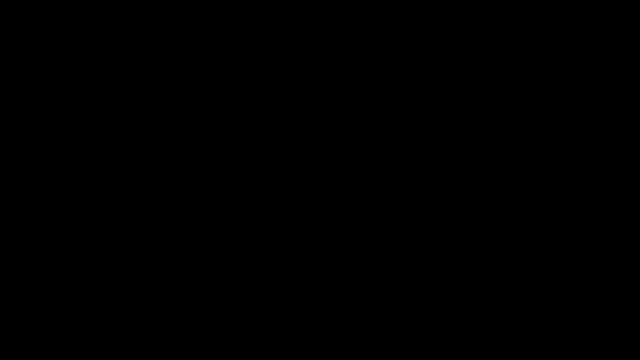 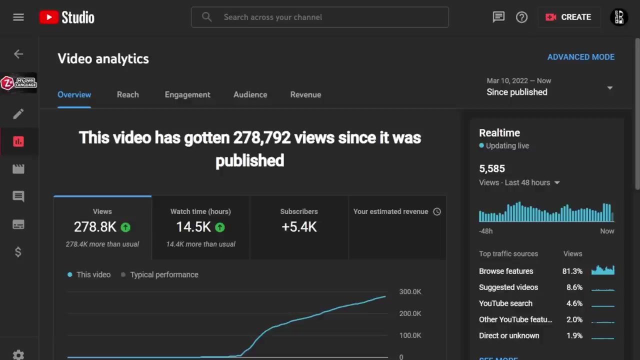 Name made before is 16 bits, not at all confusing, don't complain. in the comments I borrowed this idea from one of my friends, Doorbellprog, Before I begin. thank you so much. My Zsharp video has an incredibly huge number of views and my channel went from. 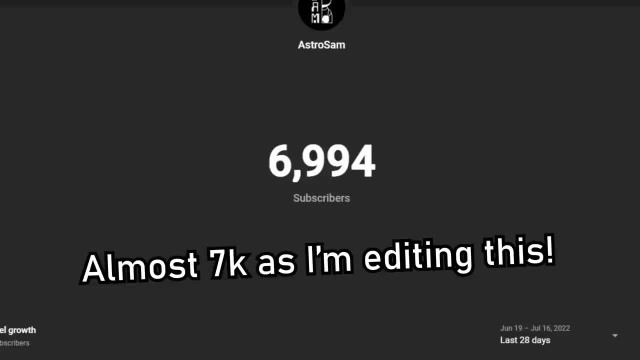 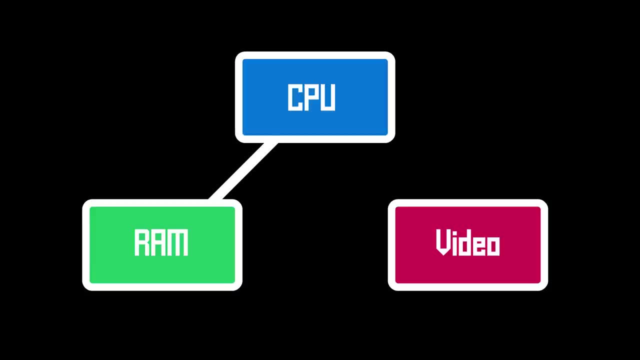 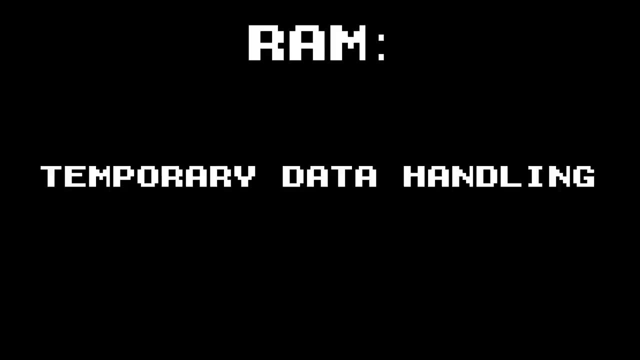 under 400 subscribers to over 6,000.. So once again, thank you, and let's get on with the video. My computer can be broken down into a few important components: The CPU, the RAM and the video circuitry. The RAM is for temporary data handling If the computer needs to keep data. 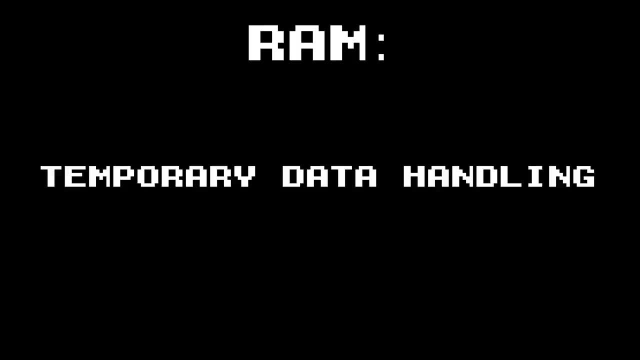 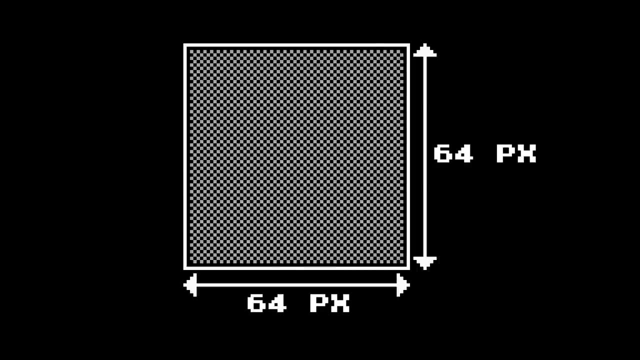 but perform another task first. then it can just store it in RAM. It has 65,000 memory locations, each of which stores a 16-bit. The display is an LED screen. It's attached to dedicated video hardware which handles pixel rendering and the CPU which handles processing data and executing. 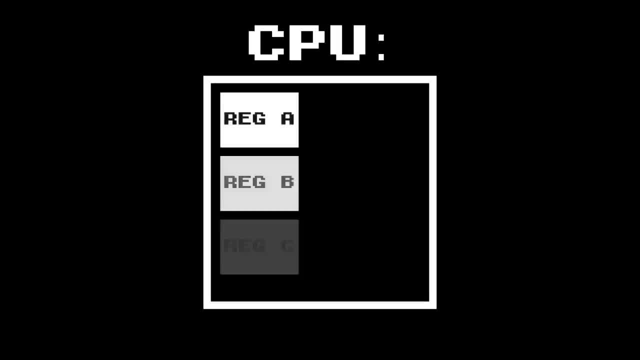 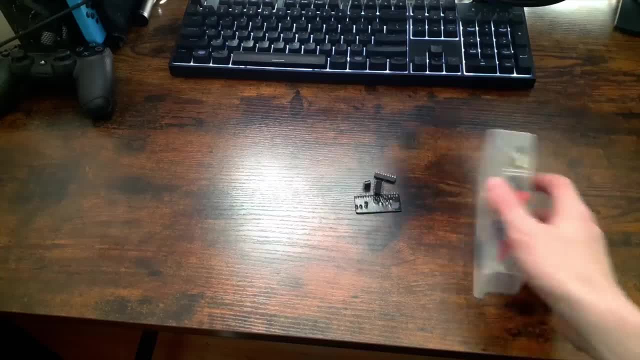 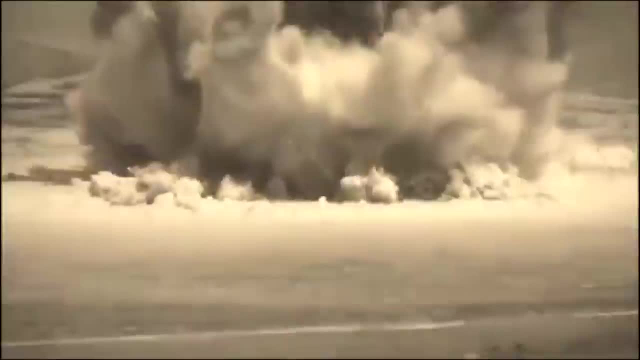 instructions Inside the CPU are many things like the registers, the multiple counters for keeping track of instructions and the arithmetic logic unit. Now, before rushing to just throw together a bunch of components and transistors and capacitors and chips and stuff like that into one horrible mess, let's actually design this thing. 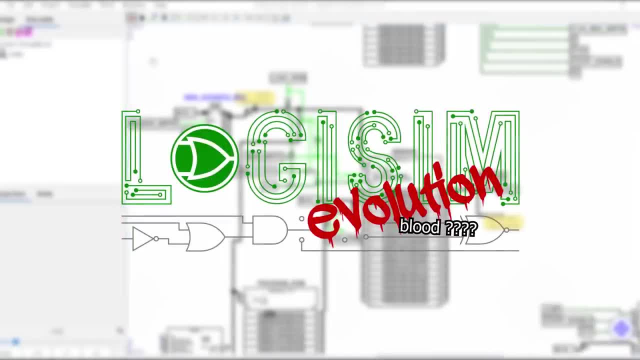 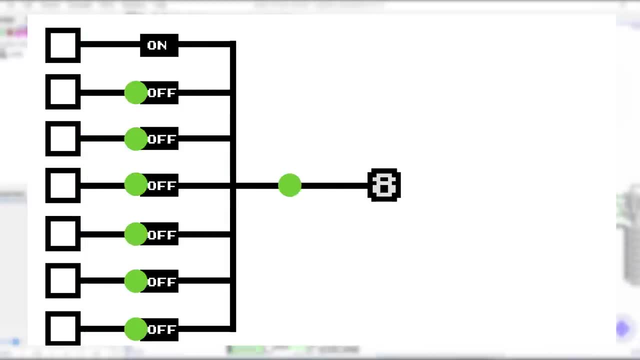 So I decided to use Logisim for the design and simulating the CPU realistically. The actual CPU is fairly simple. It's basically a lot of different on and off switches which allow different parts of the machine to execute and move memory and data, which then produces the desired output. Let's first go over the 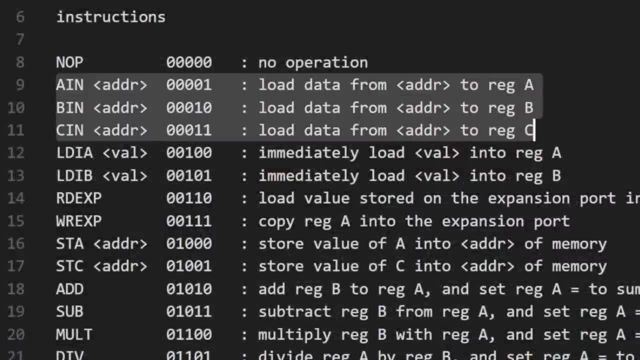 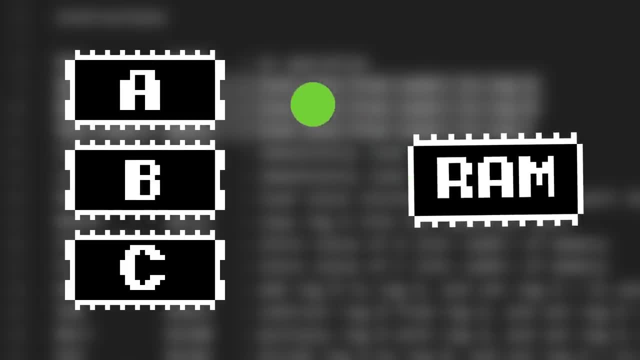 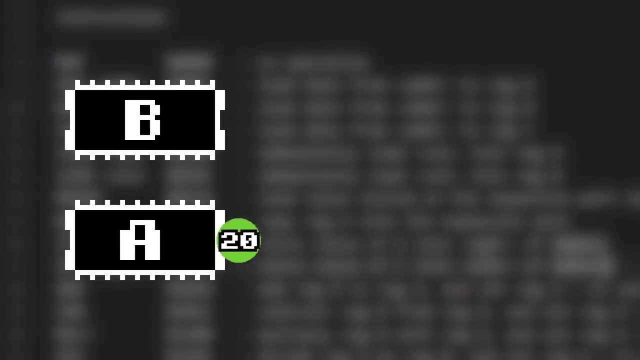 instruction set of the computer. The computer has 23 different instructions. The first three instructions are for reading from a memory address into one of the three general purpose registers, A, B and C. The second two instructions are for loading integer values directly into A and B. 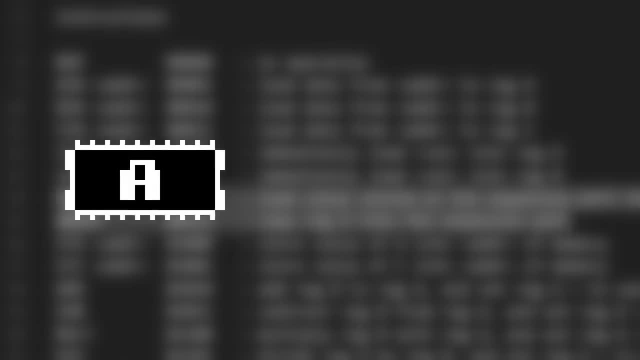 Next we have the read and write instructions for reading and writing to the expansion port on the computer. There's a 16-bit port which ties directly into the bus and is available for any device to use. Next we have the store commands, which store the value of either register. 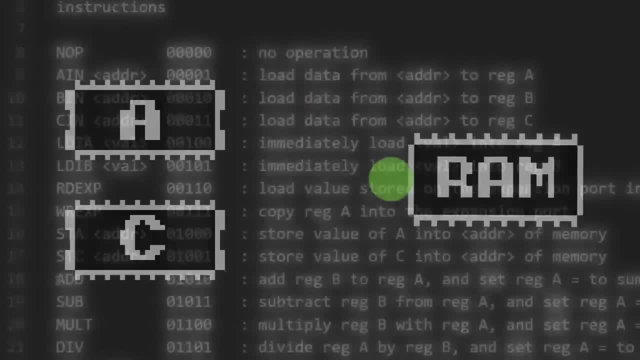 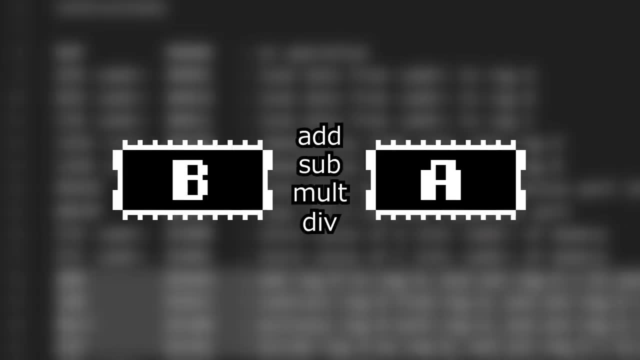 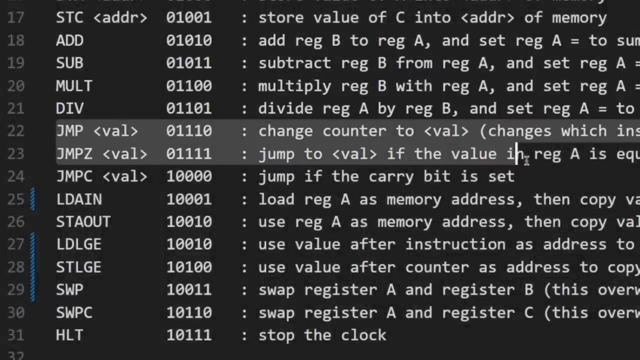 A or register C into an address in memory. Then have some arithmetic commands such as add, subtract, multiply and divide, which apply one of those operations onto the A and B registers. There are three individual jump commands which are used for. 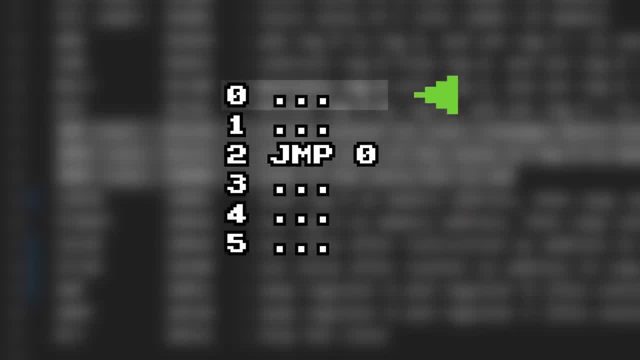 different reasons. The first one is used to unconditionally jump to whatever address in memory. The second one is jump if zero, which checks if the previous arithmetic operation equaled zero. If that is not the case, then it will simply skip this jump command. There is also 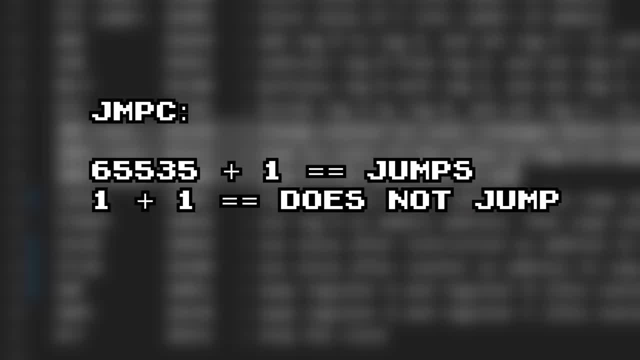 jump if carry, which will only jump if the previous operation had a carry. For example, if you add two numbers and they're large enough to have made it overflow, it would only jump if that is true. Otherwise it would also skip this one. Here's some more load and store commands. 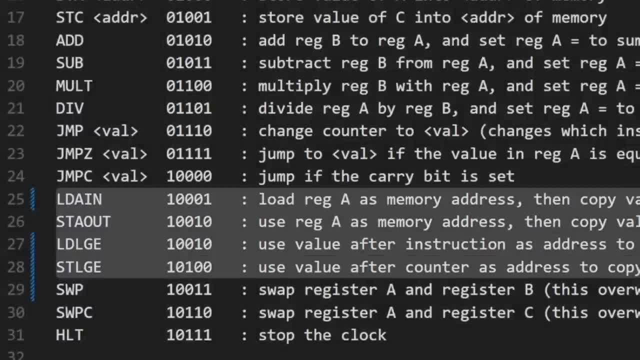 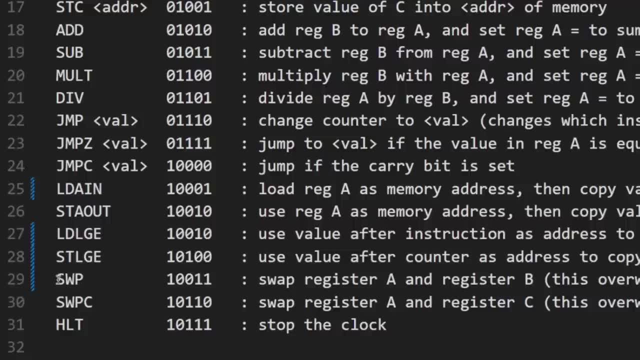 which are just used to access higher values that can't fit inside of 11-bit, which is all that the instruction register can hold, along with the actual instruction bits. Next, two commands are for swapping registers. Next we have the load and store commands, which are used for swapping. 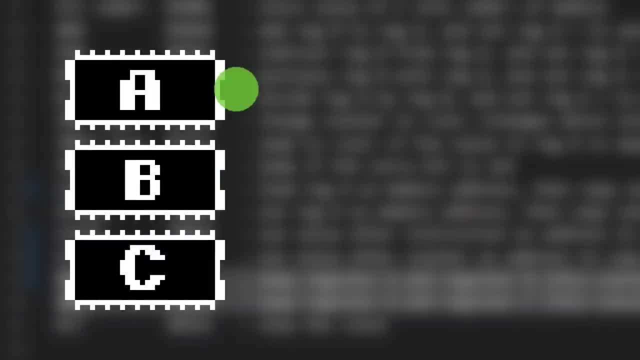 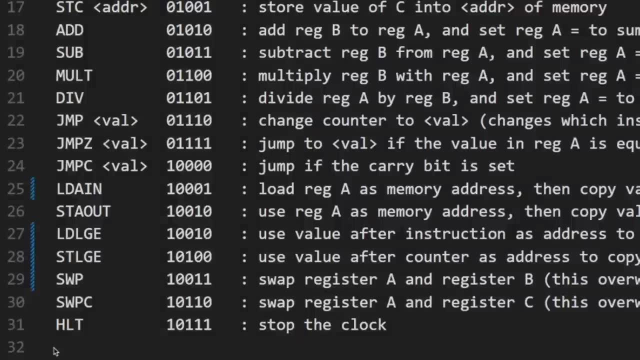 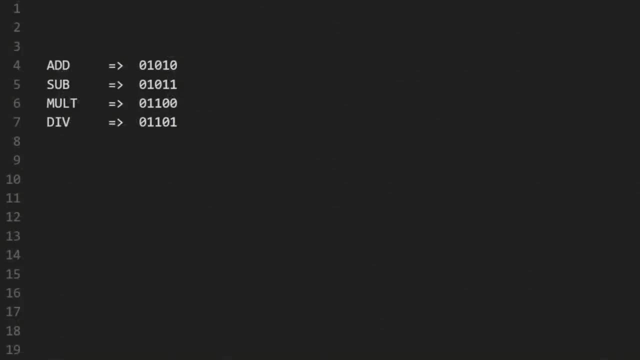 register values. The first one swaps A and B and the second one swaps A and C, And the final command is halt. This simply stops the clock and doesn't allow the computer to execute any more instructions. Assembling the instruction set is actually very simple, You see each instruction actually. 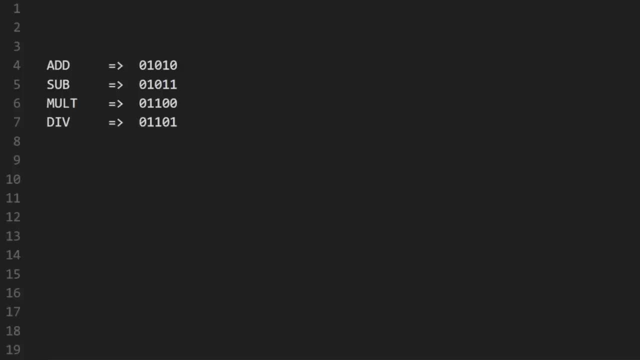 corresponds to a binary value and that's just its index. So if it's the first one, then it's number one, If it's the second one, then it's number two, and so on and so forth in binary. This binary instruction code only takes: 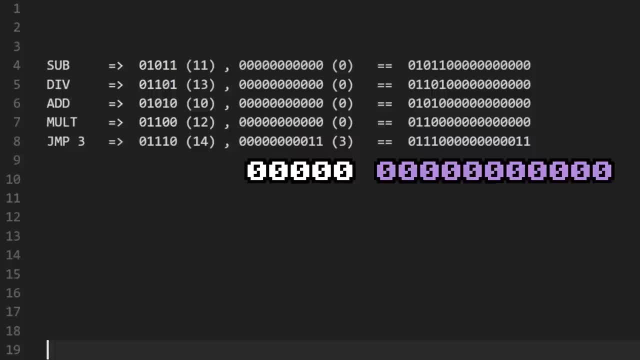 up five bits, So we have another 11 bits out of the 16 available to use for anything we want, such as a memory address or any other arguments that might be used for the command. So all the assembler does is replace all of these values with their binary values. 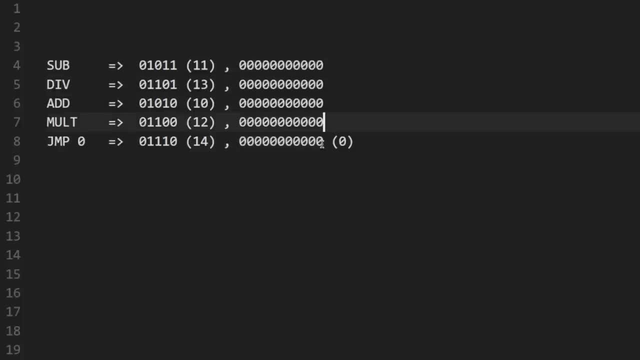 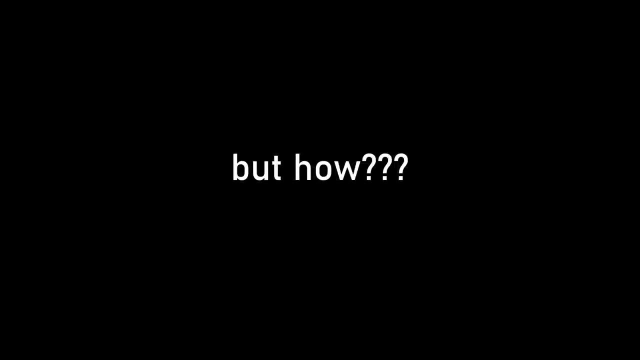 and convert all of the arguments into their binary values as well. Now you may be wondering: how exactly do these instructions tell the computer what to do? Well, these instructions don't exactly tell the computer what to do. Instead, they're each. 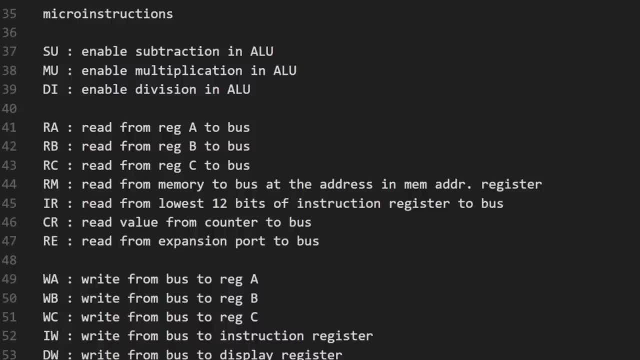 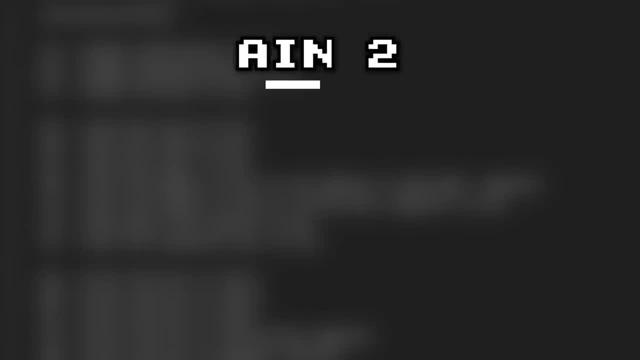 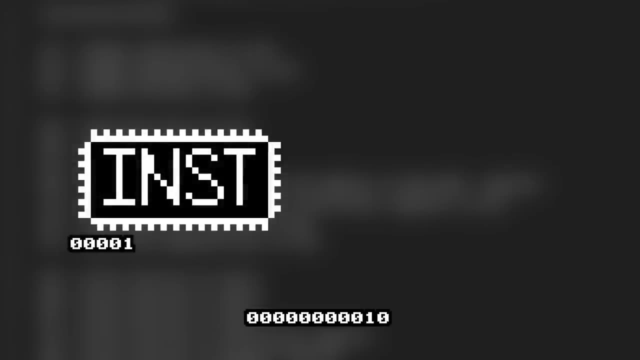 comprised of something called micro-instructions, which is an even more broken-down version of what the instruction does. For example, the first instruction is a-in and the first step that a-in is executed, it will read from the instruction register: This just gets the address that we're 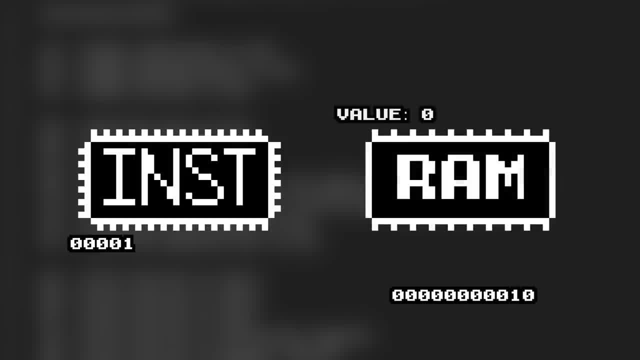 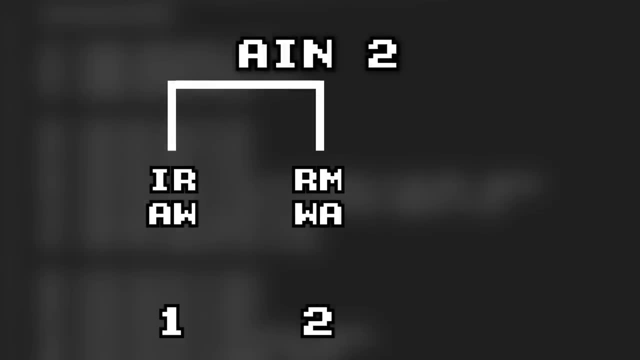 talking about and trying to read from, And then it writes that address into the address register. This changes where the RAM is pointed to, so now, instead of pointing to wherever it was before, it points to the address that we're talking about. After both of those are done, in the next step. 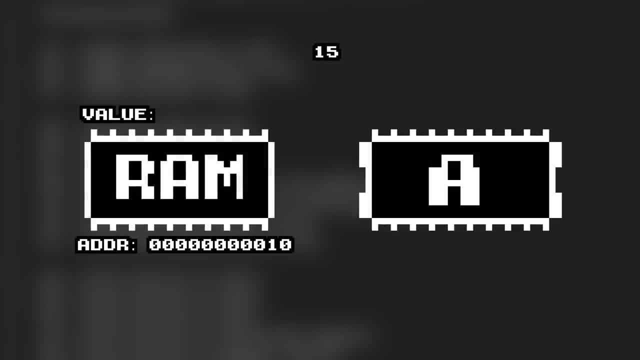 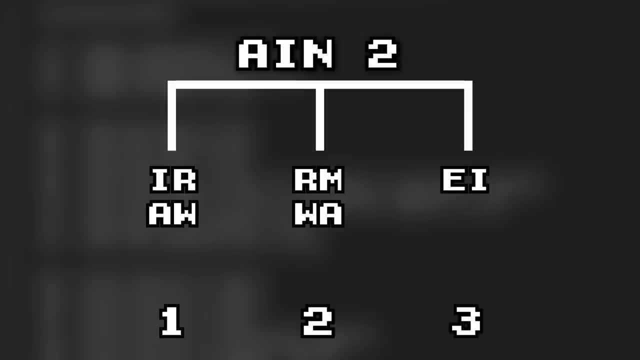 it will read from that memory location and it will write the value into a. And the final step, which is actually the final step in every single instruction, is the micro-instruction called ei or end instruction. That just signifies to the computer that there's no more steps to be executed, so it can. 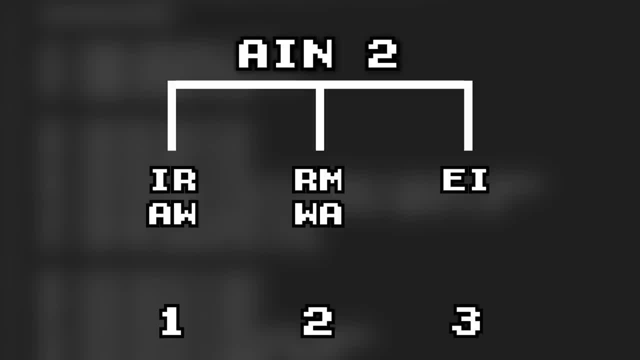 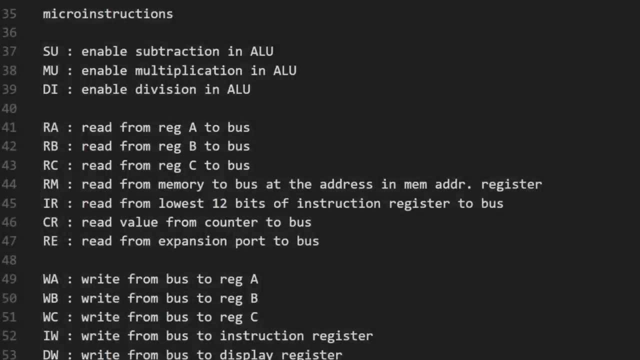 end execution for that instruction and move on to the next one in the program memory. In total there are 24 micro-instructions which in combination can be used to create all of the normal instructions above. Now you may wonder how we're able to get all of these micro-instruction outputs. 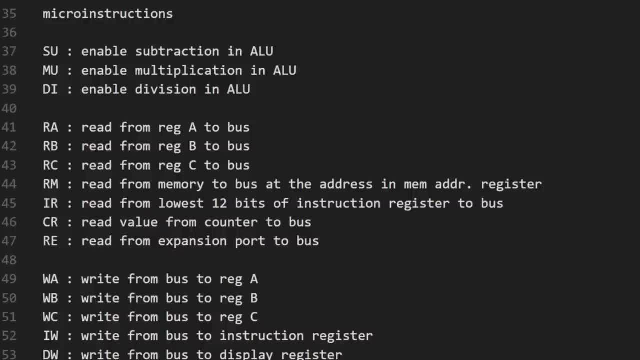 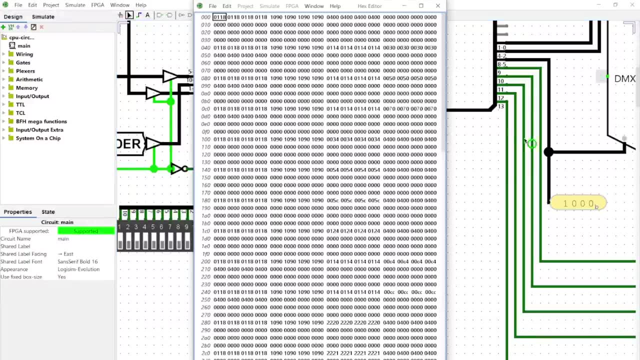 from a large number of instruction inputs. Well, that is actually done through a lookup table or, in this case, a ROM. This ROM is pre-written with all of the different combinations of input bits and then the value is fed out, and then the values are fed out to the other inputs. So, if you want to, 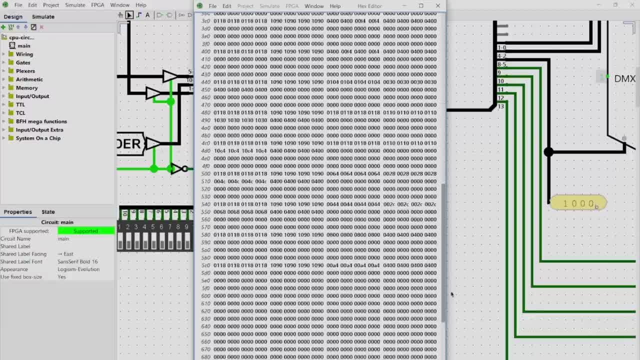 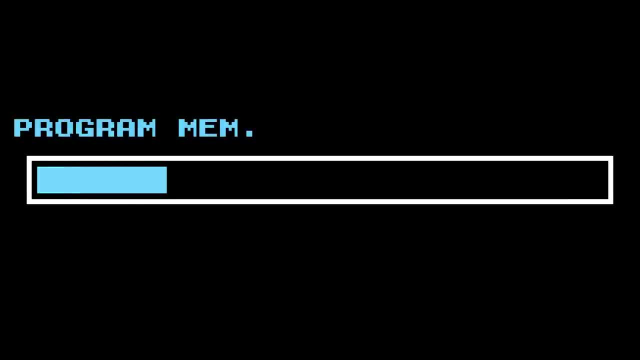 get all of these into a number of demultiplexers, it turns on and off the desired micro-instructions. The memory is laid out like this: The first 25% or 16,000 words are dedicated just to the program. 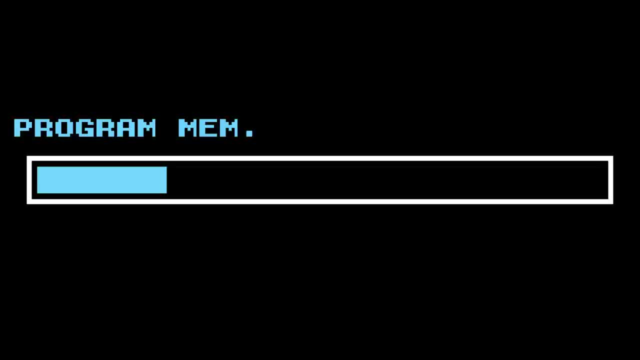 This is all of the instructions that tell the computer what to do in each program. The next 144 words are just for character memory. This is where the video circuit will read from in order to know what letter or symbol to display on screen. This is where the video is located, and the other words will appear on screen at the end of the program. 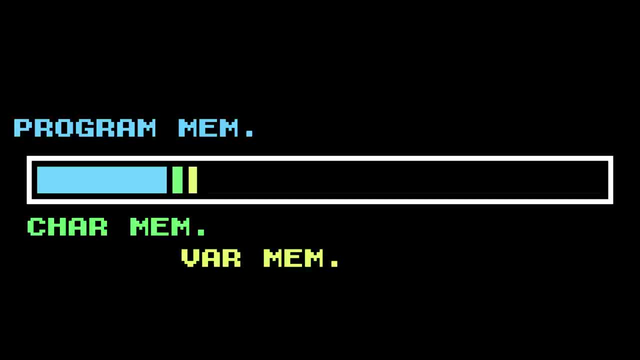 The next 128 words are for variable memory, which is an allocated spot for the compiler where it knows there is free memory and it can put new variables there and they shouldn't get overwritten Between the variable memory and memory location 61,000,. this is general purpose. 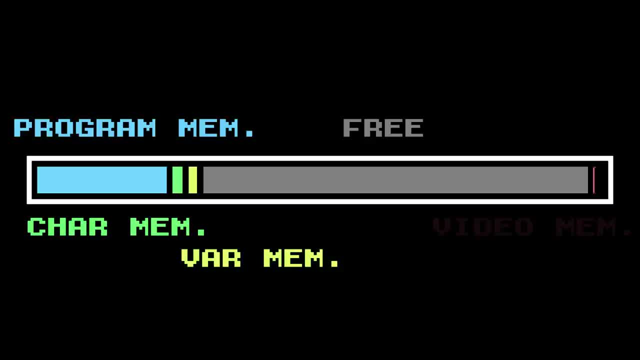 memory that can be used for any reason. Finally, from memory location 61,000 to 65,000, or 4,096 words, that is dedicated to the video memory And you can use it to work with your students. video memory, which is where the video circuitry will read from in order to know what color. 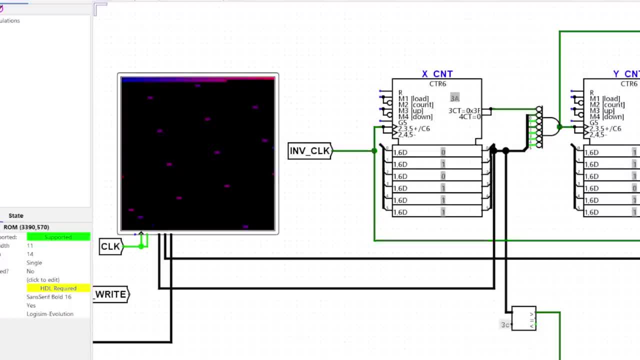 each pixel is Something that makes up a surprisingly large portion of this computer is actually the video circuitry. This here is Logisim's video emulator, which allows you to input a number of pixel RGB values and write pixel colors to the screen. 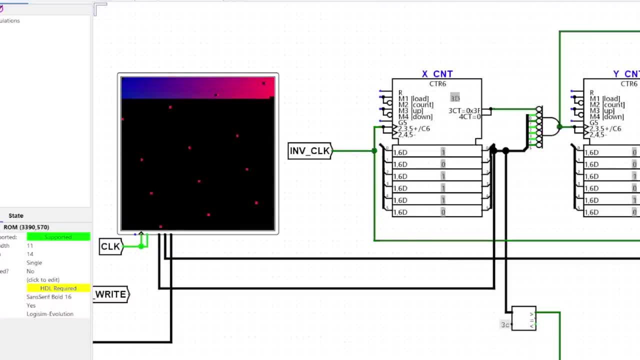 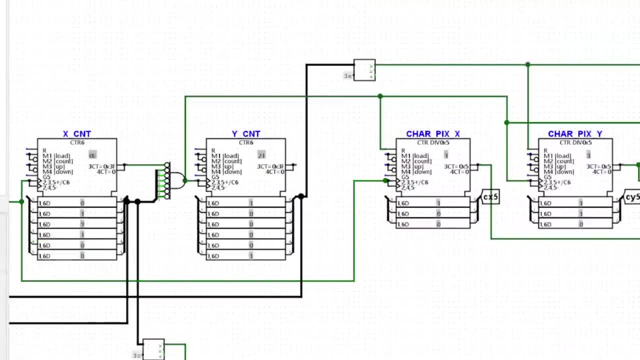 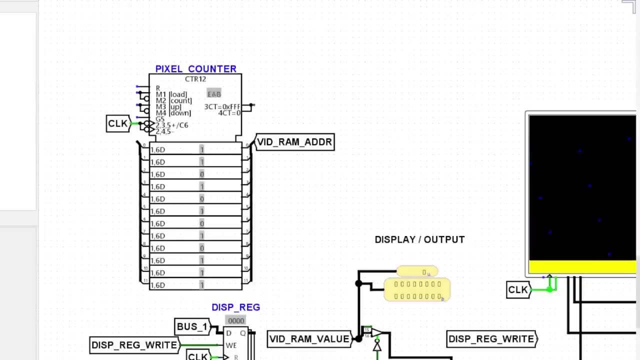 Connected to it is six individual counters which increment on each clock pulse or when different requirements are met. These ones over here are for incrementing in the character RAM. This tells the computer what letter or symbol it should write. And this one over here is for pixels, which tells the computer what pixel color it should. 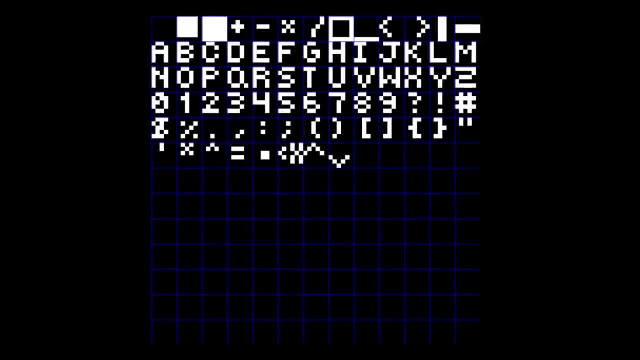 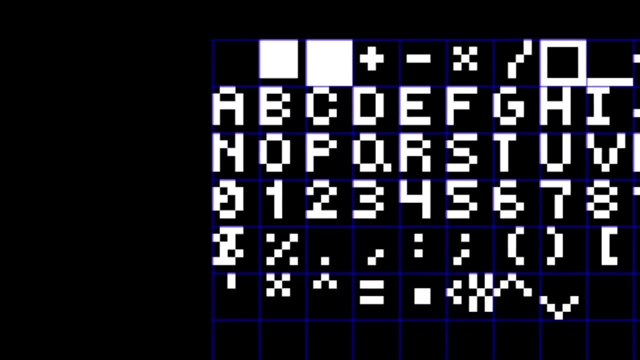 write from the video memory. Now, getting back to the characters, there's actually an entire character set that I made for this computer to allow it to easily display symbols and letters. This is what it looks like: That all fit inside of a six by six grid. 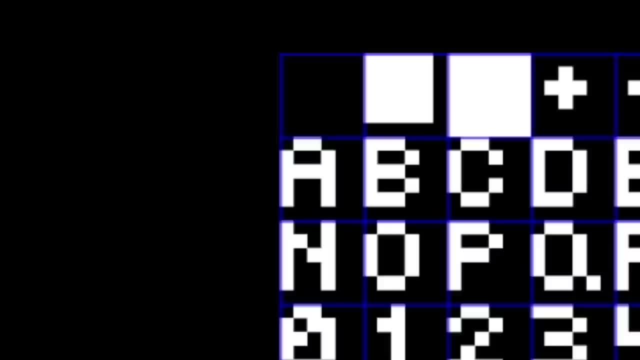 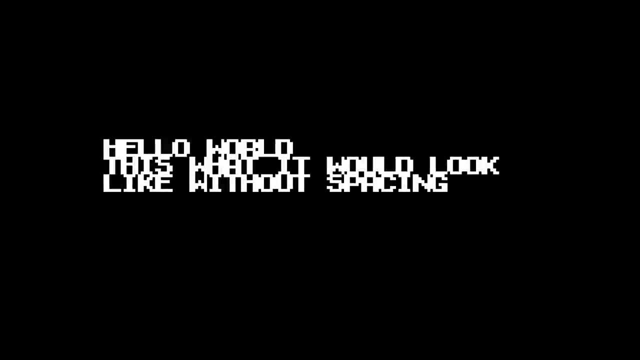 Now, most of these actually only take up five by five, because I allow a one pixel space on the bottom and the right. That's because the computer does not automatically add these spaces, so all the letters would look all crammed together. Some of them, though, actually do utilize this space because they're meant to be used as 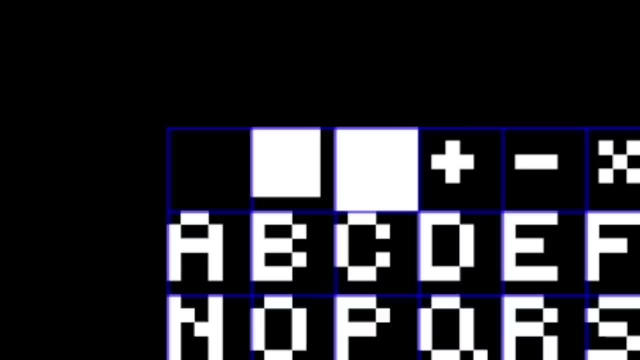 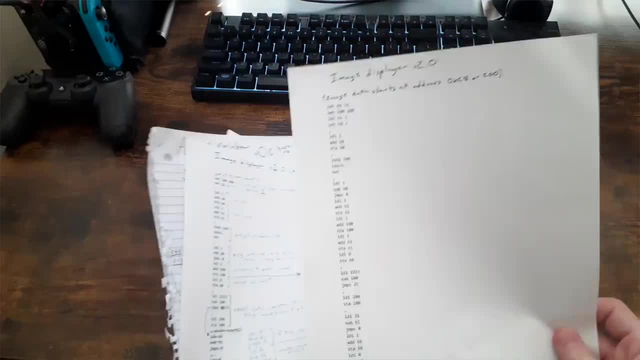 more of a symbol or graphics character which wouldn't normally be used accompanied by normal text. Now let's get on to how I wrote some programs. Initially, I just used the instruction set and wrote programs like that, although it became very, very complicated. And I couldn't figure out how to do that. So I just used the instruction set and wrote programs like that, although it became very, very complicated and I couldn't figure out how to do that. So I just used the instruction set and wrote programs like that, although it became very, very complicated and I couldn't figure out how to do that. 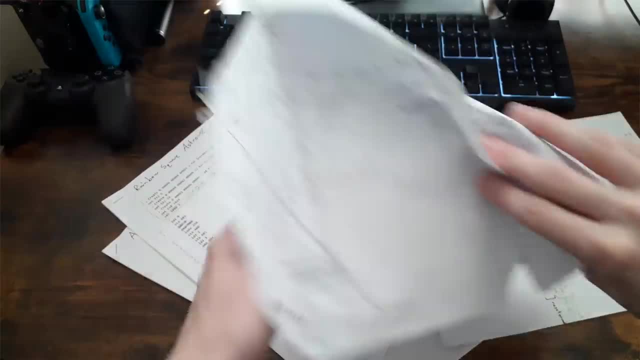 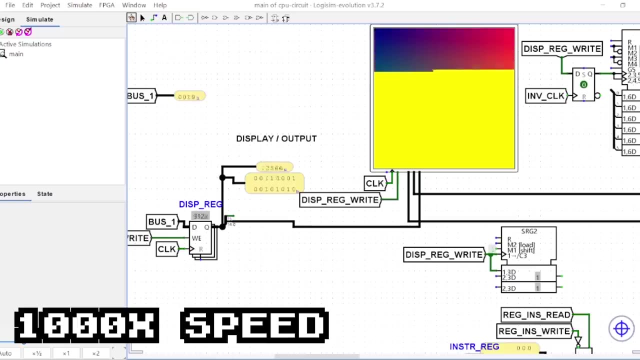 I was going to figure out some bugs sometimes and I'd spend hours just working on one little program, For example. look at this program right here. As you can see, it just draws a rainbow square in accordance with the x and y coordinates. 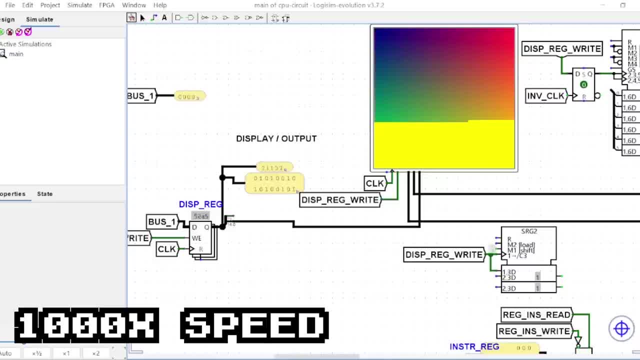 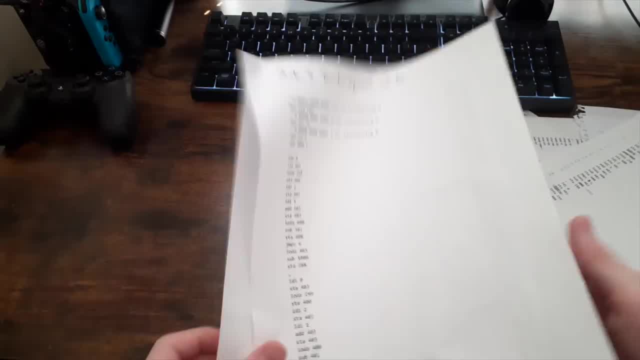 Well, this one took three different revisions and I had to print them out in order to make enough comments and be able to debug it easily. Here are all the different versions, until I finally got it working, And this wasn't even a complicated program. 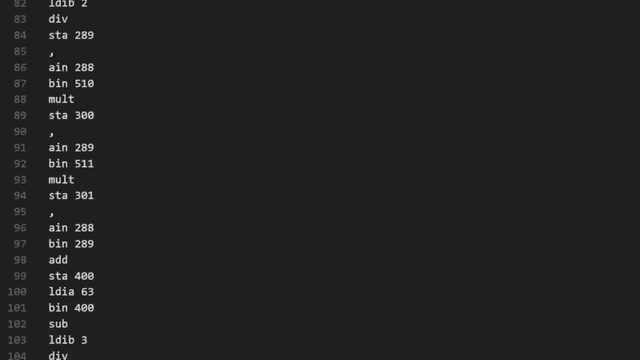 All it did was write out to the pixel coordinates pixel coordinates the x and y values. It would be very difficult to make any sort of game with this, so I decided that I needed to actually make a compiled language which would compile into this. 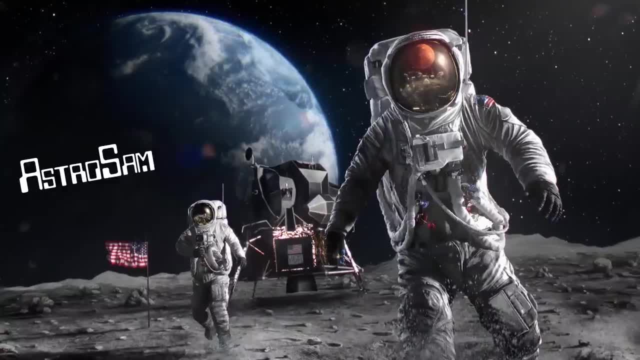 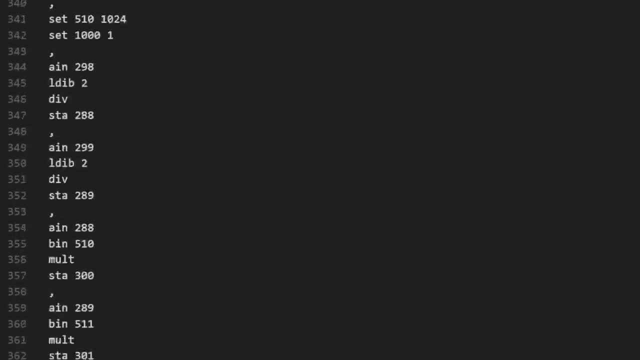 It's called Armstrong, suggested by Baddock. Hopefully you can you know. see the reference. Now, we've already been through this once before, but let's go over a bit more about what compiling really is and how this language is different from my last one. First of all, this one will 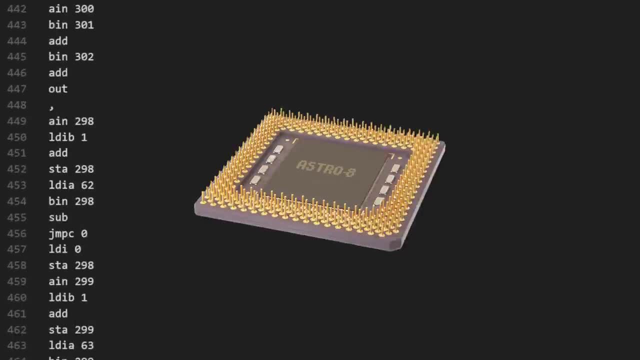 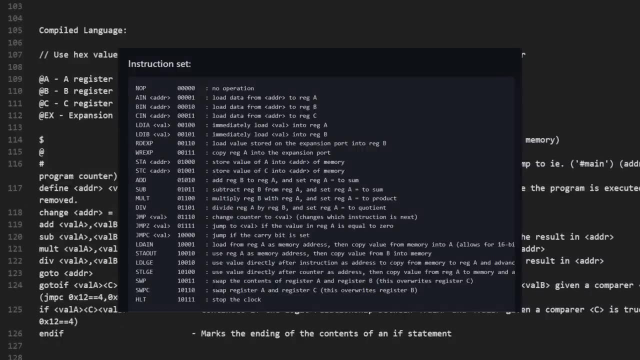 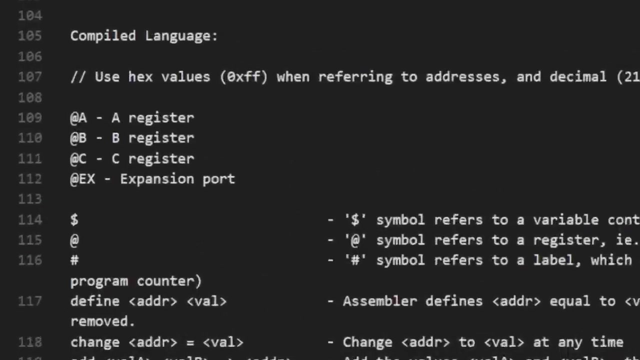 not work on your Windows or Linux computer. This one only works on my computer, my processor to be exact. The 24 different instructions in the instruction set I was able to narrow down and combine to create this right here. You can now easily change register values using the at. 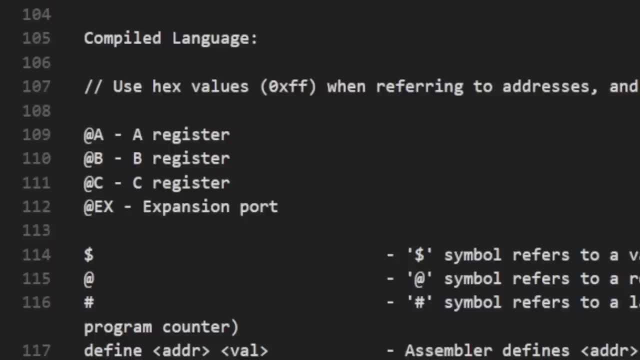 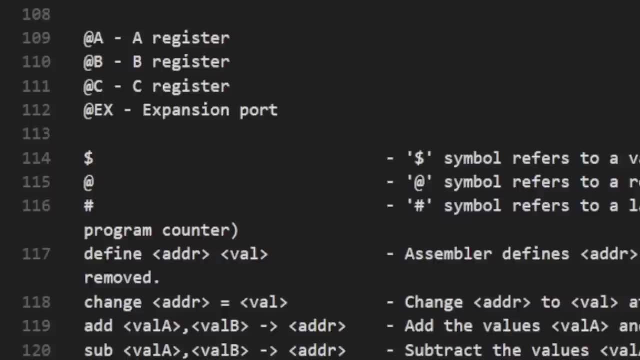 prefix and a, b, c or the expansion port, because the expansion port is also counted as a register. just to make it a bit easier, There are also now variables using the dollar sign prefix, which the compiler automatically allocates memory for. 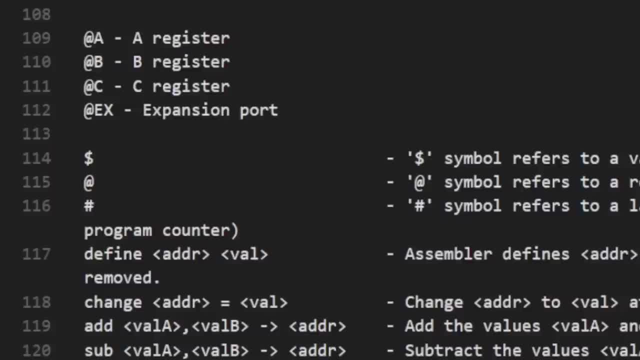 and that way, you don't need to use exact memory addresses in order to access data. And there's also the label, which is using the hashtag prefix. This is a place where you can easily jump to in your code, and that way, you don't need to use specific line numbers. 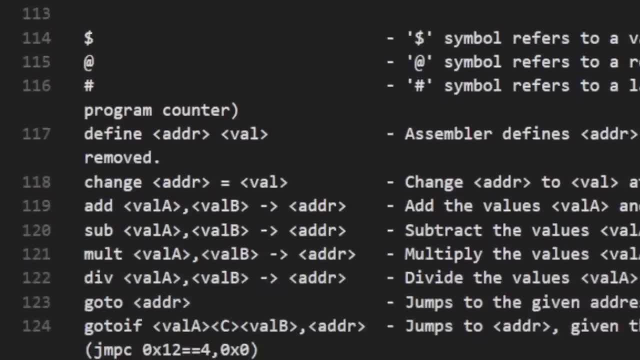 which are dynamic and change. There's the define command for defining a memory address. There's the change command for changing any value equal to another value. There is the add, subtract, multiply and divide commands which do those operations on two input values. 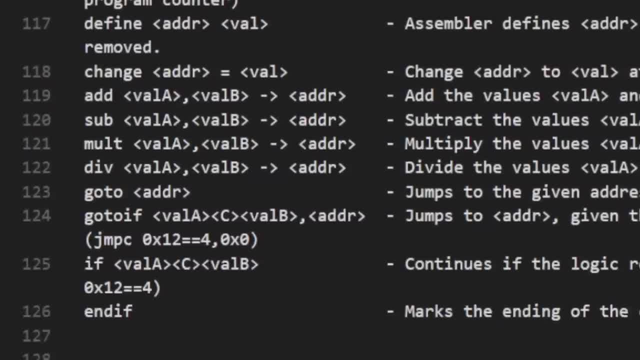 and then put it into the output value. Then there's the go to command, which goes to a specific line, number or label. There's also the go to if statement, which only goes to the line number or label if the comparison between its a and b values is true. And finally, there is the 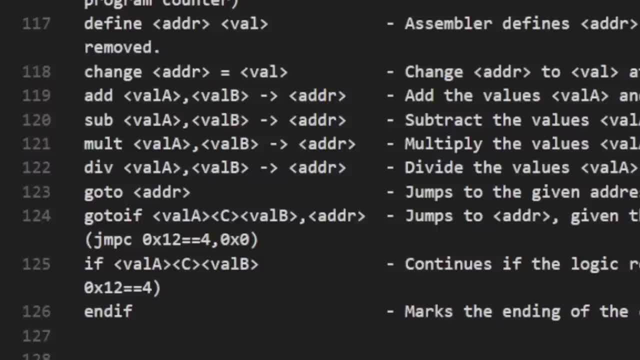 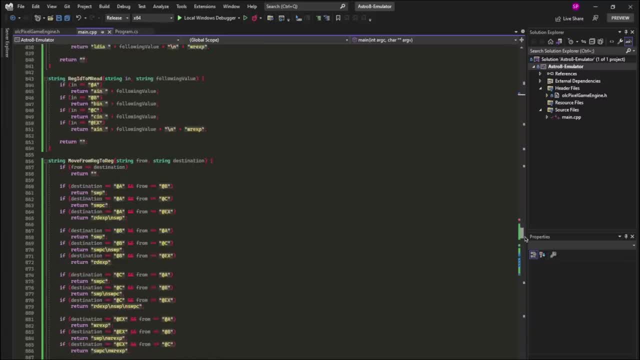 if statement, which is just like the go to if statement, but instead of jumping if it's true, it just continues inside of the if statement. And then there's the add subtract multiply if it is true. So in C++ I built a compiler which would compile it all into the instructions. 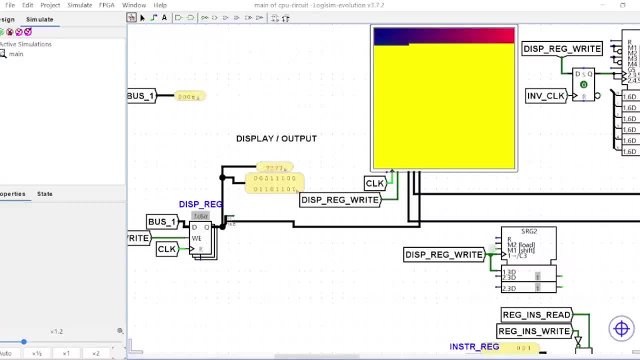 And it looks like this when we compile it Now. if you remember the rainbow square demo that I showed you in logic sim, then you'd know that it is not very fast. In fact, it is much lower than one frame per second, And that isn't actually the fault of the program. The program is perfectly fine. 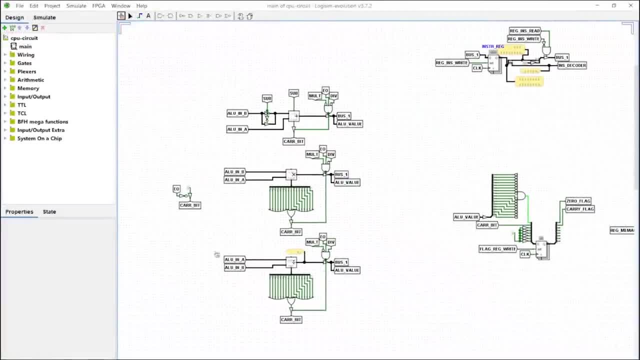 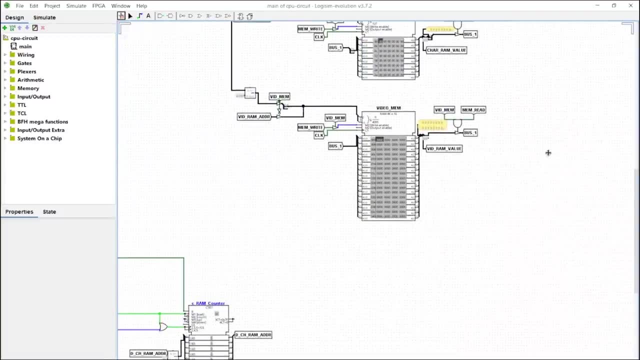 as it is. It's actually because logic sim needs to simulate all of the different logic relationships and logic parameters, And that's why it's so important to have a logic sim that's able to navigate And that actually takes a lot of processing to do So, in order to actually 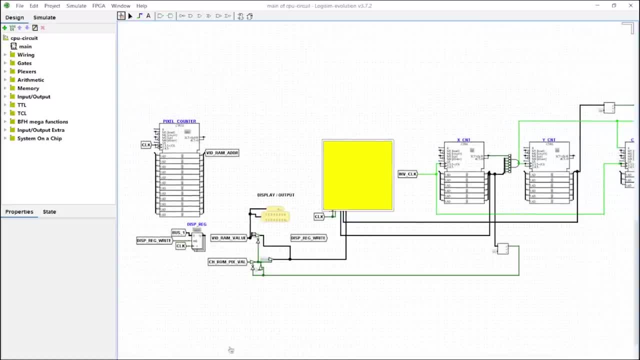 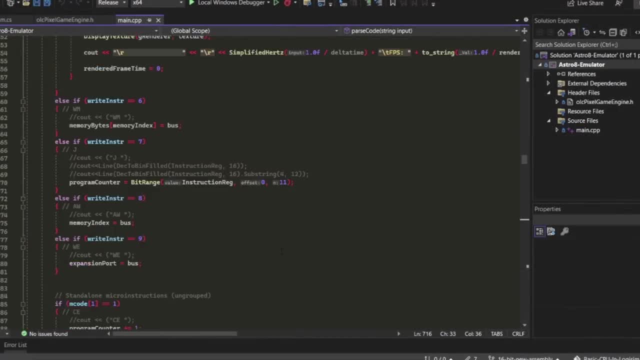 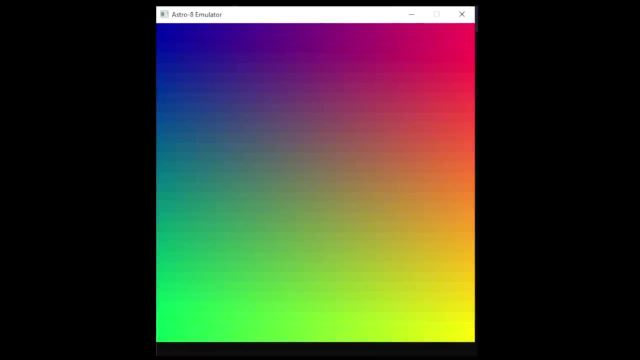 run something at full speed. I decided that I need to make an emulator- So I also use C++ and STL2 for the graphics- and built a working emulator that could correctly process all of the instruction sets and correctly respond as if it was the actual hardware running the code. 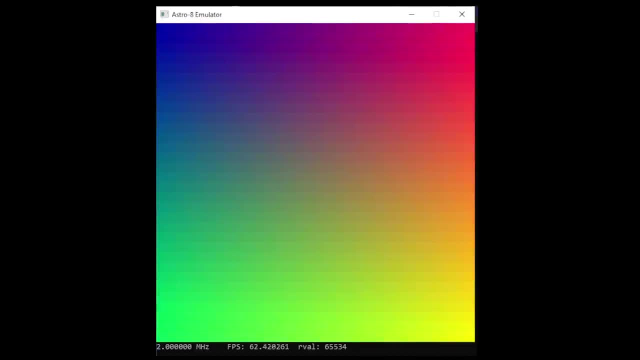 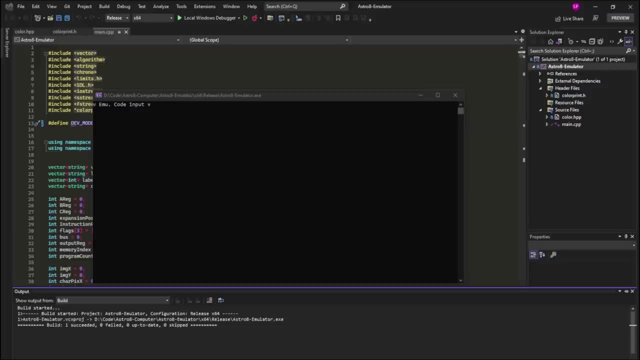 So it runs it identically to logic sim, although it runs it at thousands times faster. So to test out the different circuitry and parts of the system, I made a few different programs which would allow me to debug and make things better or change them as 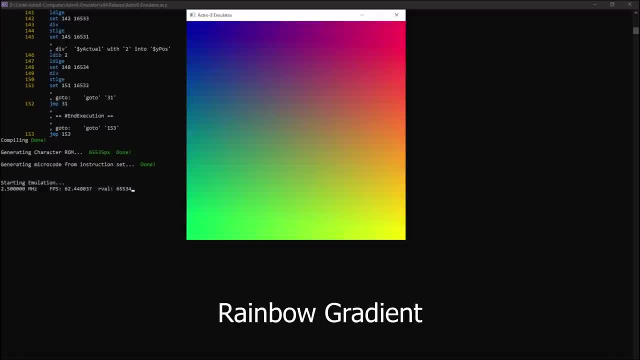 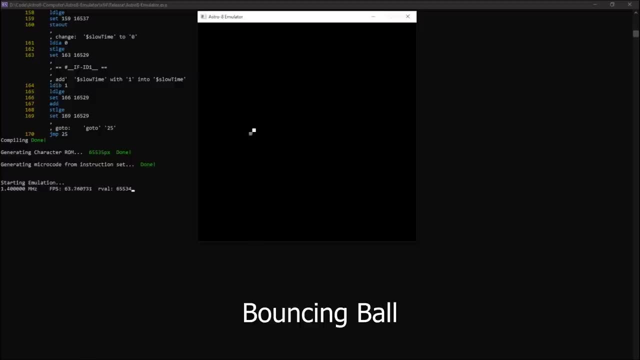 I saw fit. So here are a few of the examples that I made, And you see, this one, the ball bouncing. Well. that one, well, what do you think I'm going to use it for? I decided I was going to make pong. 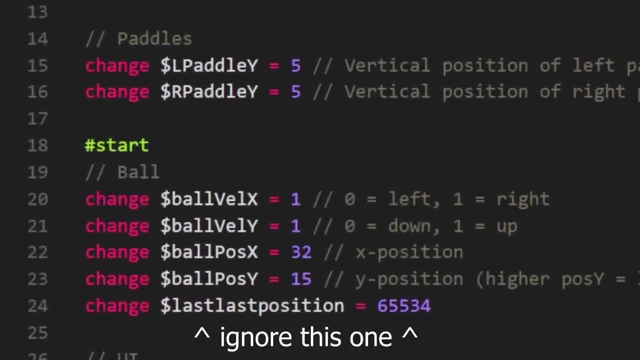 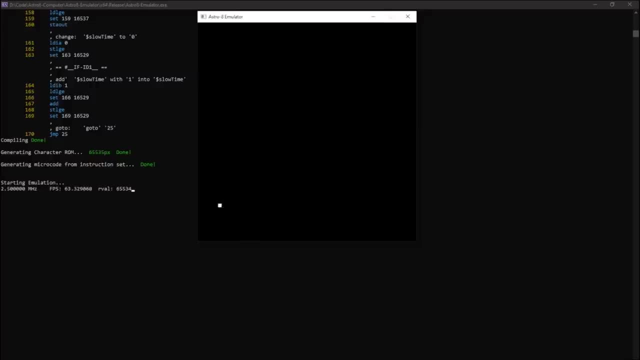 The ball has four different variables about it. It has the X and Y position, as well as the X and Y velocity. It moves diagonally until it hits a wall. If it was on the left side of the screen or the right side of the screen, then it will swap its X velocity. So 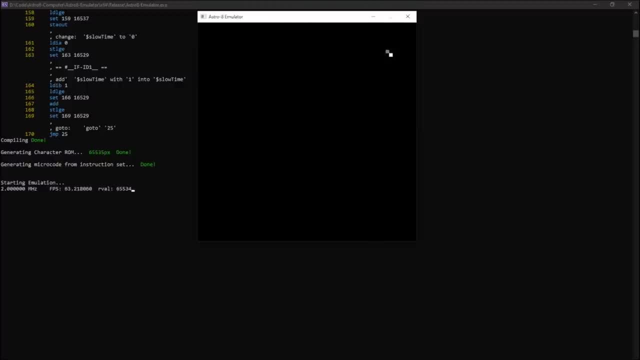 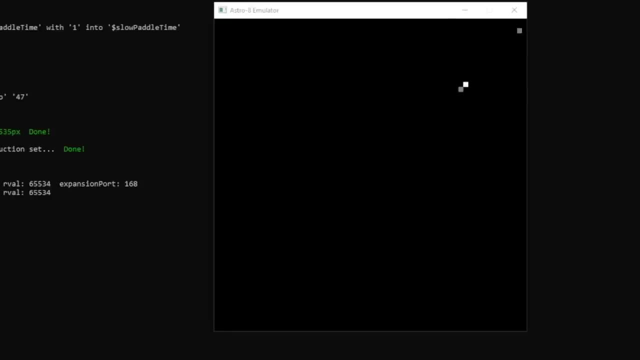 it looks like it bounces off of it, And same with the top and bottom of the screen. it swaps its Y velocity. So to make this work for pong it needs to turn off the left and right walls. So the ball now goes through them and responds in the center of the screen. Now, this is not all that pong is. 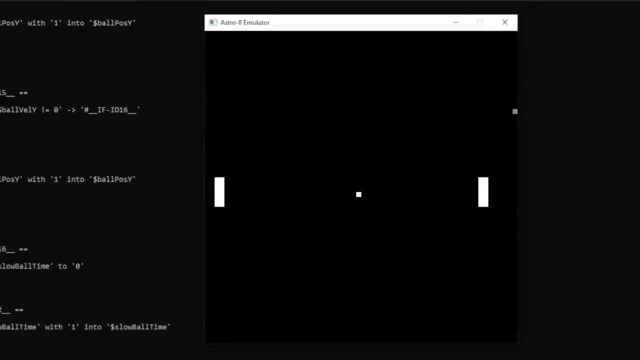 of course. So I also made the left and right paddles. Those paddles are actually characters, This one, to be exact in the character sheet, And that's because it would take more processing time to actually write all of those pixels to the screen using bitmap mode. 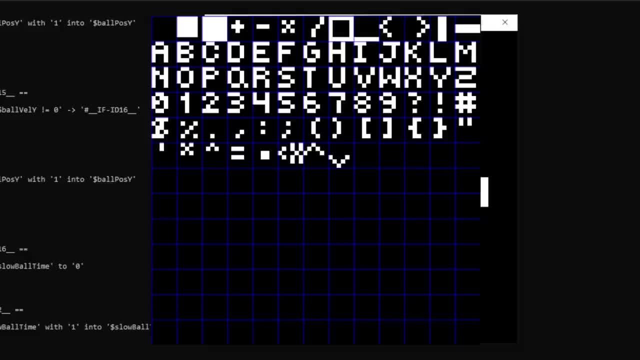 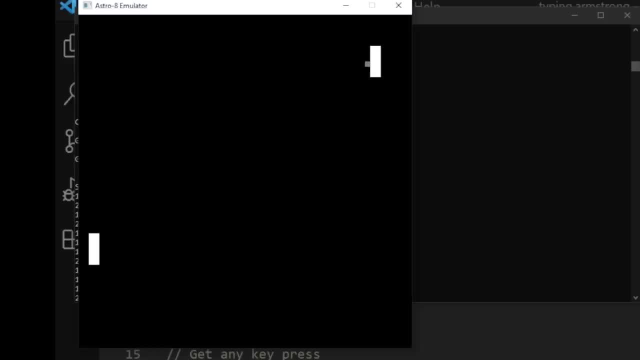 Although, as you can see, all the characters are confined to this grid on the screen, So it does look a little bit blocky when you move up and down. So, then, what I did was some very simple rectangular collision, which just checks if the ball is inside of either of the characters. Now, 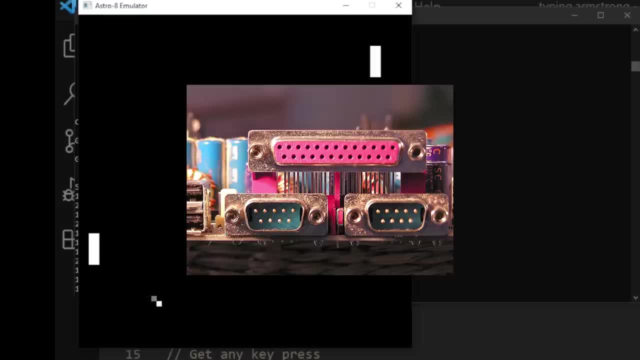 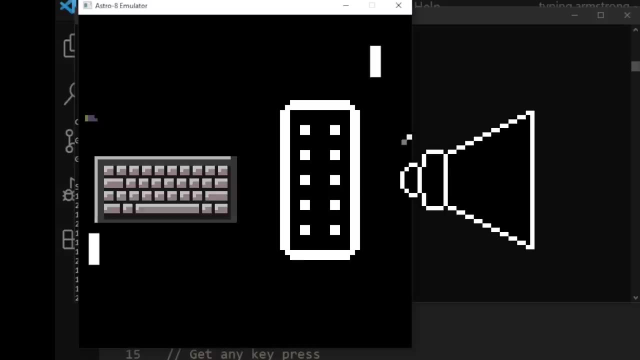 the paddles actually need some movement And luckily that's where the expansion port comes in. You see, the expansion port can be used for many, many different things And in this program I decided I want to use it for a keyboard. So I made a mock keyboard circuit emulator. 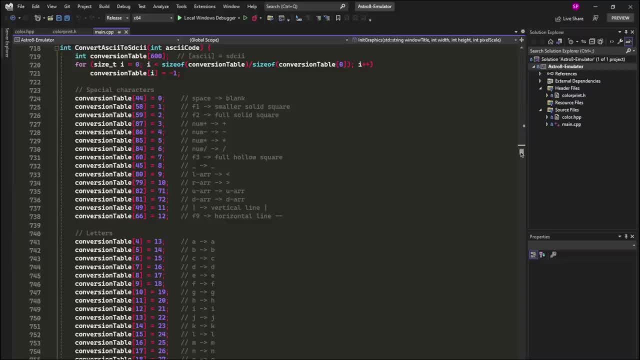 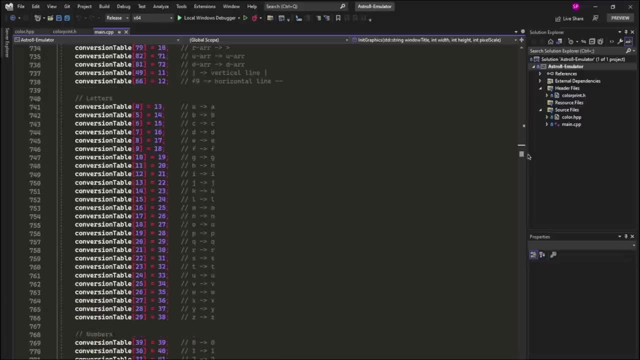 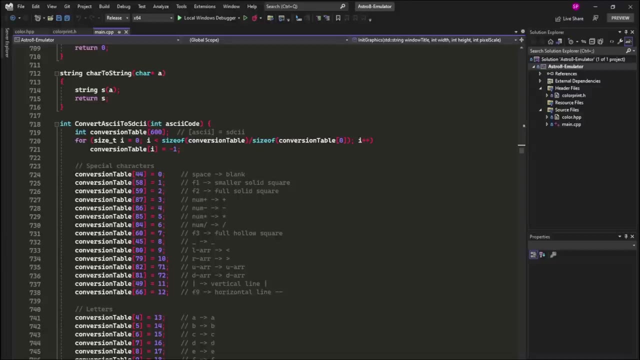 which converts the ASCII character keys on a normal USB keyboard into my special character mode, which uses different indexing, And so inside of the pong program I can just check if the expansion port- which in this case of course is a keyboard- is equal to the W and S keys for up and 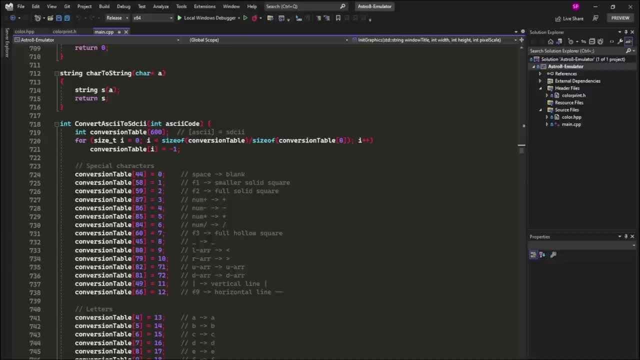 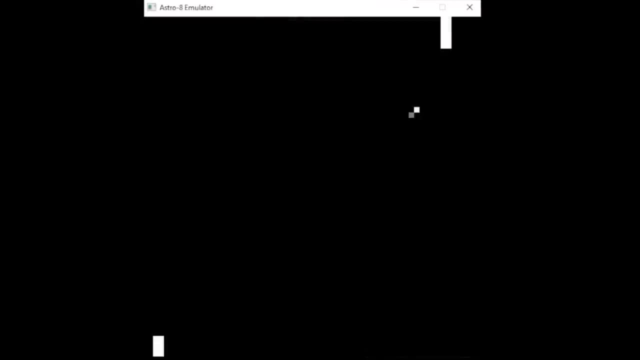 down or the up and down arrows for up and down for the right paddle, And then I can just offset the character in memory accordingly. Unfortunately, since this code is run hundreds of times per second, that means that the instant that I press one of the movement keys, it actually moves the 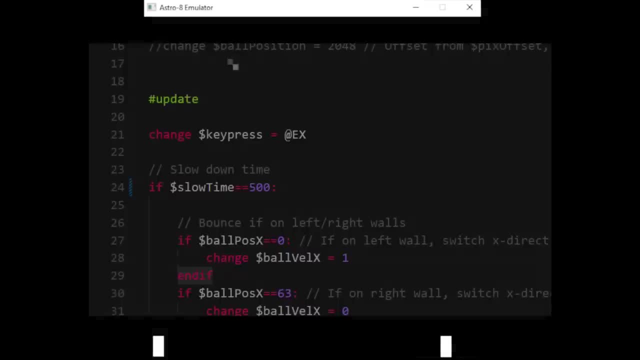 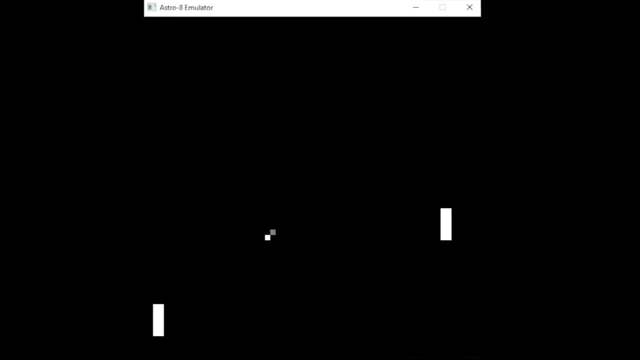 paddle all the way to that side of the screen and there's no wait time. So instead I hacked a little way inside of the code which allowed it to only register a key press once I've released the key or longer time has passed, meaning I can hold down the key, although it'll move a lot slower than 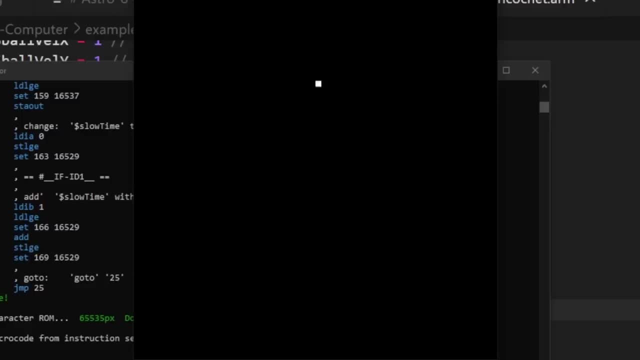 before. I also had to do something similar with the ball while I was still making the ball demo, because the ball would move very fast across the screen. Using the program didn't have much computing to do, and so the ball therefore bounced very quickly across the screen, But I just limited. 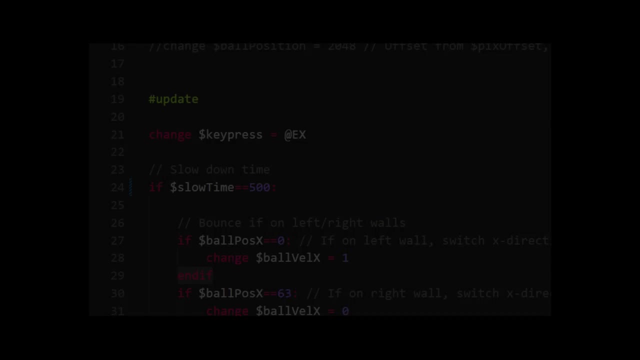 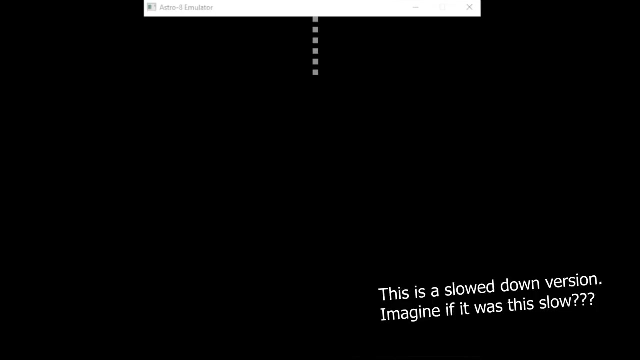 it to only change its position every couple hundred cycles. After I had all of that done, I made the net in the middle of the screen. Very simply, it was just a loop that drew gray pixels on the screen every 128 pixels from the last one. Now the final thing, of course, is keeping track. 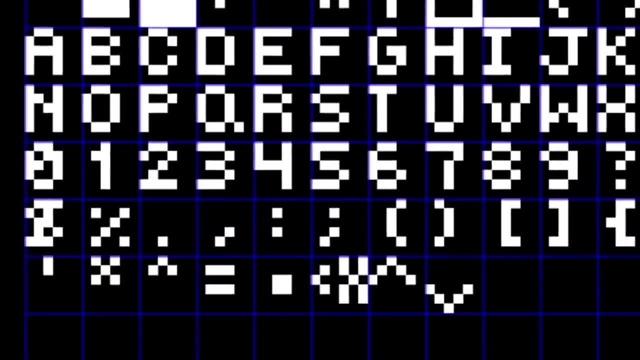 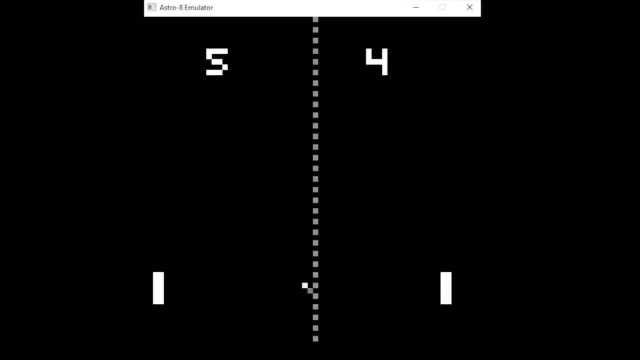 of the score. Luckily, I obviously didn't have a lot of time to do that, so I just did a little bit of math. I obviously made numbers in my character set, which means it's very simple to just display a simple score number from 0 through 9 using the player's score, which increments every time the 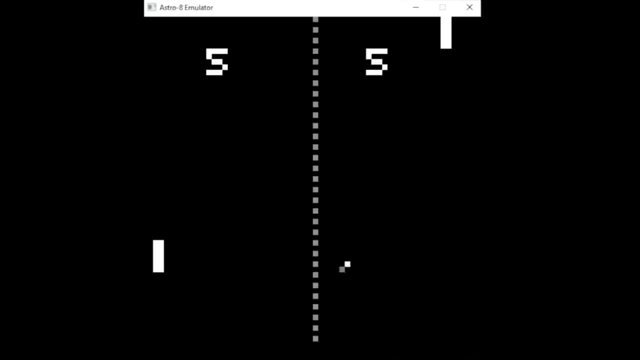 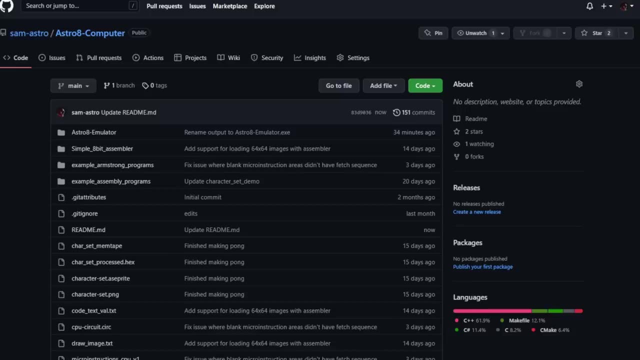 ball goes past the opposing player's side. Upon reaching 10,, they win and the game is reset back to the beginning and they can continue playing Once again. this project is open source on GitHub, so you can go ahead and go to the link in the description where you can try it out.